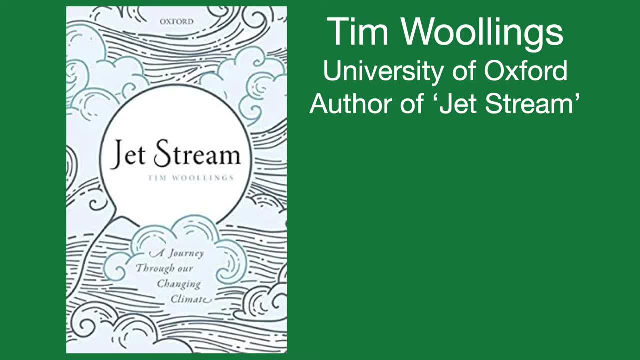 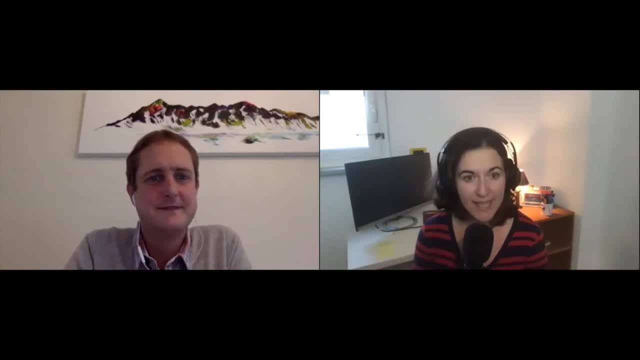 Thanks, Tim, for joining me today in this episode of the Climate Academy podcast. No, my pleasure. Thank you for having me. Yeah, so you are a professor at the University of Oxford, And what do you study And how does this book fit into your research? Yeah, so I study atmospheric dynamics. 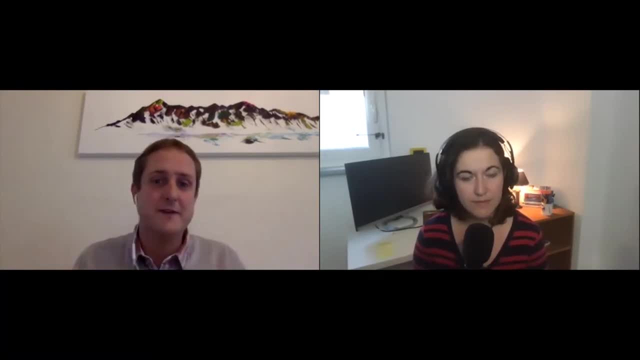 And so this is essentially to do with the kind of movement of air masses in the atmosphere. So it's the science of the kind of circulation systems of air moving around the atmosphere and also of kind of weather patterns and things like that. So yeah, this book. 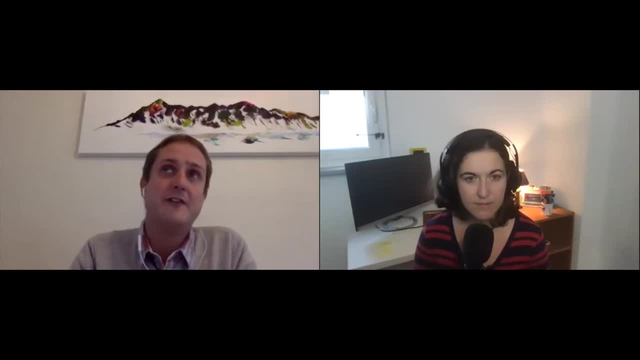 this book focuses on the jet stream And the jet is really central to lots of atmospheric dynamics. It's the kind of the big main circulation feature that you see particularly in the atmosphere, And so it's really central to the kind of the big main. 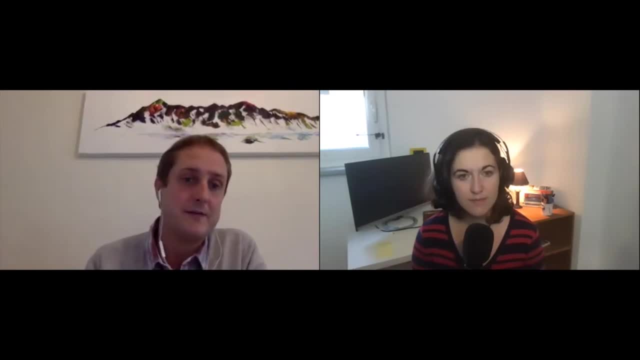 particularly in the mid latitudes of Earth's atmosphere. So it's really the kind of you know, it's kind of the most important thing. So for lots of people in the kind of you know, in the mid latitude regions of Earth, if you only, if you could only get one bit of information, 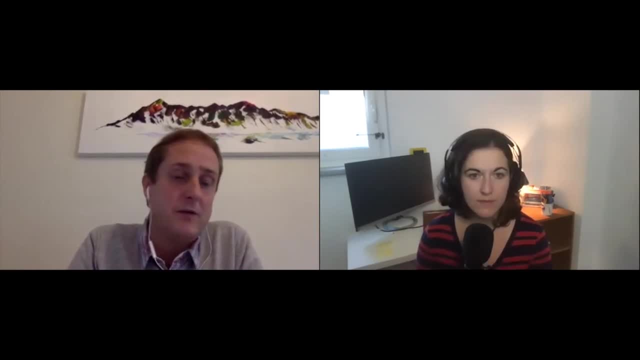 about the atmosphere and you wanted to know, you know, what the weather was going to be like then that one bit of information would very often be about the jet stream. You know, you'd want to know where the jet is and how strong it is, and things like that. And sorry, that's two pieces of information. 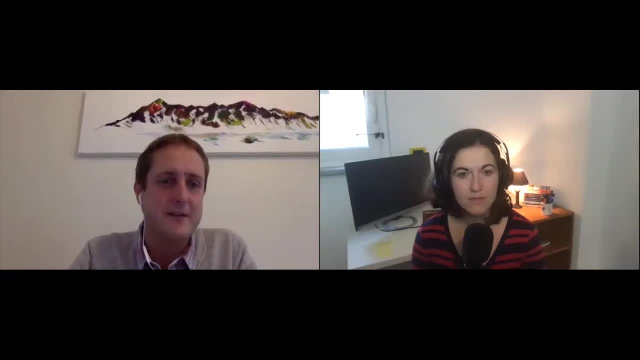 isn't it, But you get the idea. the jet is kind of the most important thing that controls our weather patterns. Yeah, so can you explain to us what is the jet stream And how does it affect us today? Today, meaning in the present day, in the present climate? Yeah, so the jet is a kind of a 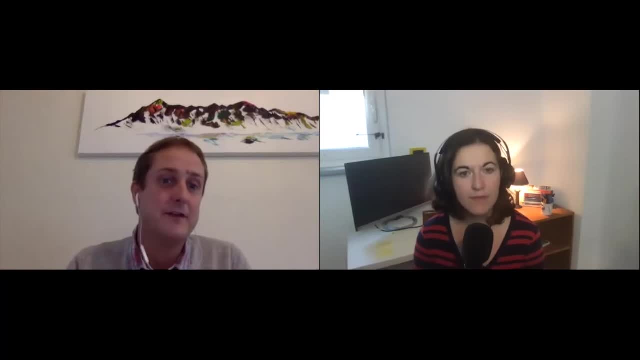 strong, narrow current of air Moving through the atmosphere. It's often, it's often mixed up with the Gulf Stream, which is which is similar but different. The Gulf Stream is an ocean current, So that's, that's kind of. 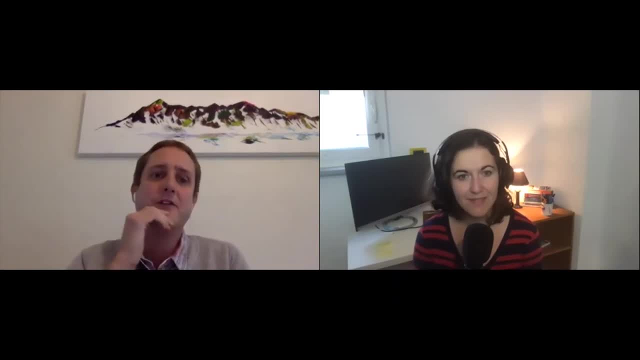 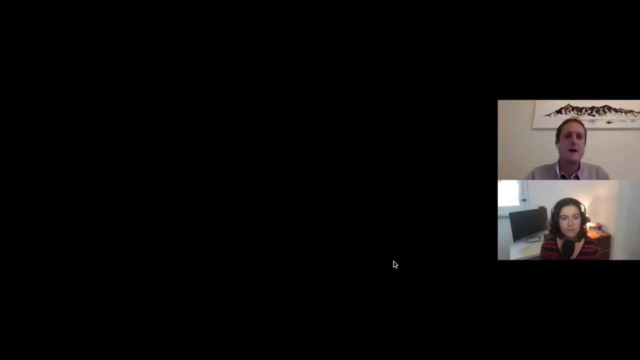 seawater moving around the ocean, Whereas the jet stream is a kind of a big current of air moving through the atmosphere And maybe easiest to show some pictures. Yeah, so I'll. I'll just share my screen, So you should be looking at a nice, nice, pretty picture of. 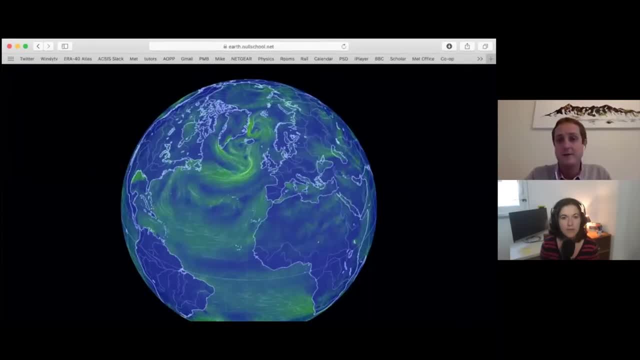 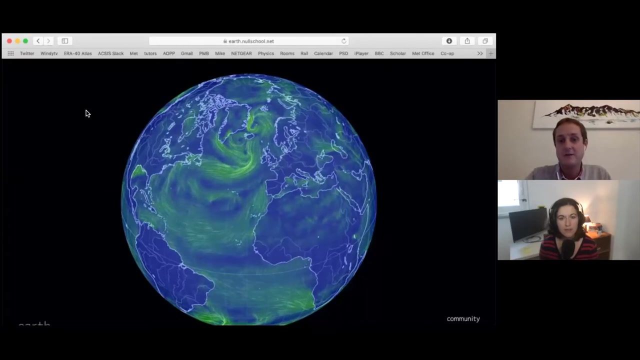 the Earth here. This is a great website that anybody can go to and browse and play with. So if you just look for earthnullschoolnet, this is a kind of a simple interface that anybody can use to kind of visualize real atmospheric data. So this is this is this is our kind of best. 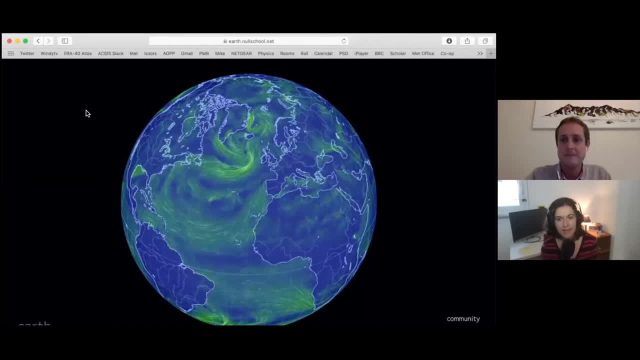 estimate. Is this coming from NASA satellites? So this comes from a, from a mix of things. So satellites provide a lot of the raw data, But then even with satellites you don't get. you don't get kind of a full picture of the atmosphere everywhere. So this is actually something called 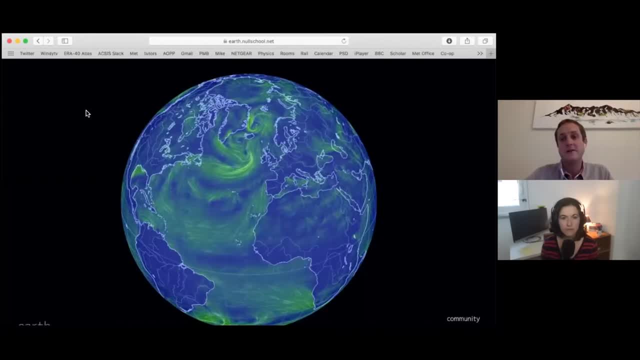 an analysis, which is where we use kind of a computer model to fill the gaps between the between the data that we have from the satellites and also from from weather balloons and things like that, And this is this is the kind of system that would be used to start a forecast. So you, 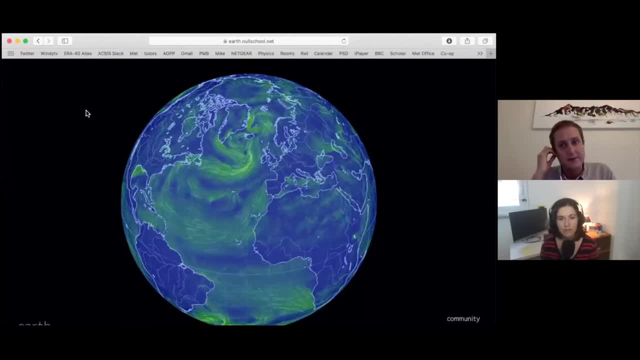 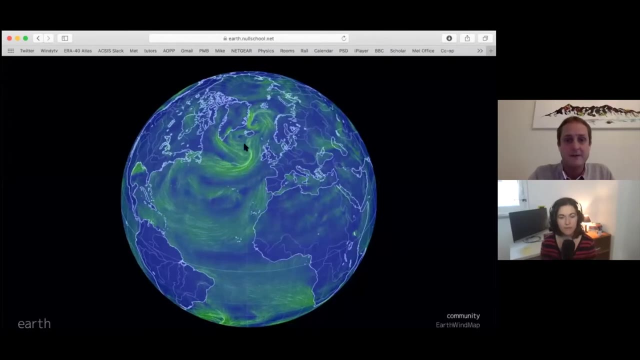 would to do a weather forecast for the next few days. you would start from this state and then kind of step forwards in time, Cool. So at the moment we're looking at the, the winds near the surface. Okay, so you can see, see some little swirly things out here in the Atlantic that are 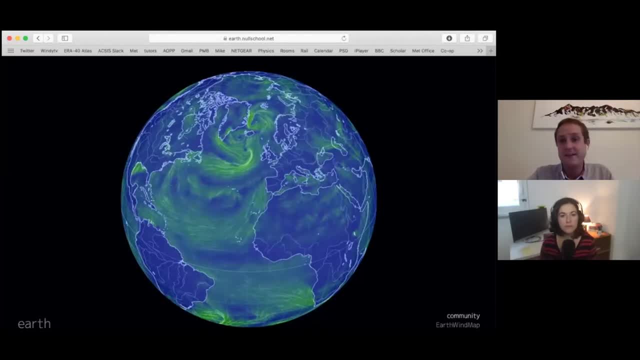 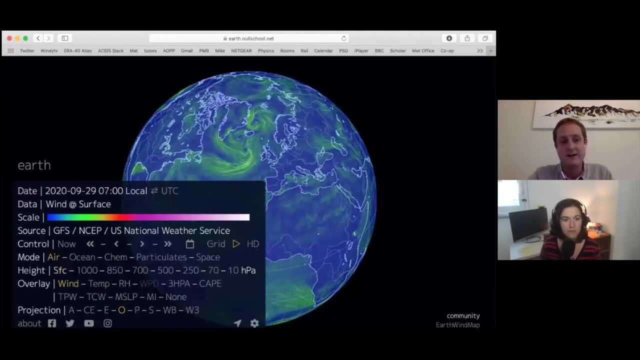 low pressure systems. But to see the jet we need to look a little bit higher up in the atmosphere. So if we open the menu here we're going to change the height here we're going to go up in the atmosphere And bizarrely that's going down in. 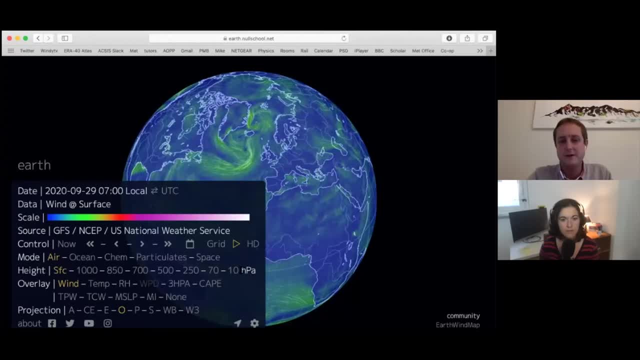 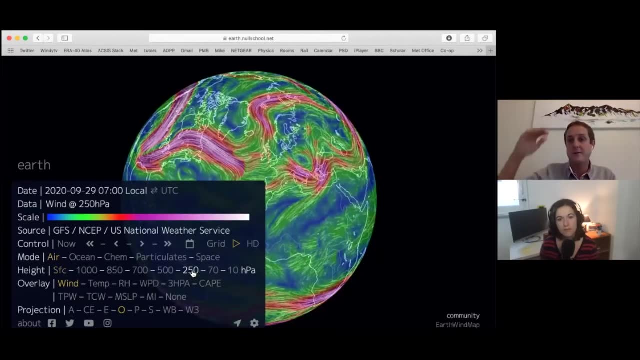 terms of these numbers. So we often use pressure as a coordinate in the atmosphere. So if we go to 250, then we're looking much higher up in the atmosphere. this is kind of like kind of like 10 or 15 kilometers up where a lot of planes like to fly, Yeah, Or at least where planes did fly. 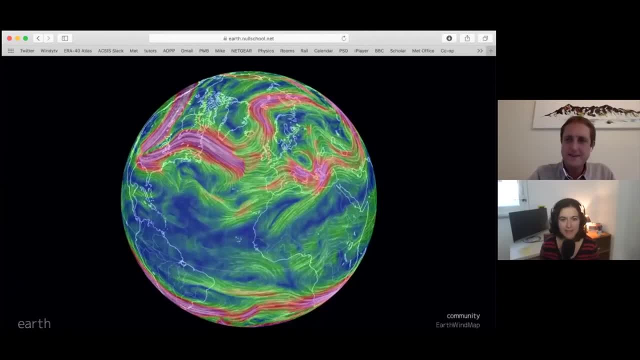 before. That's. that's also why planes from the United States to Europe are much faster then the other way around. That's right, exactly, Yep, Yep, Because now that we can see, looking up at this level, we can see that the winds are a lot stronger, right, So that the colors here and the 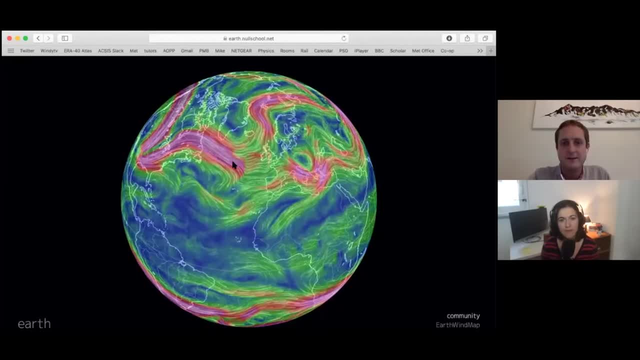 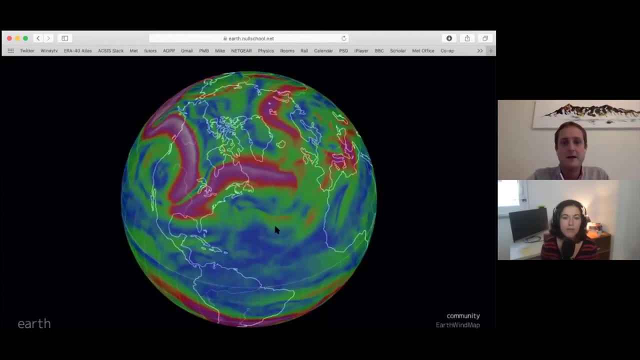 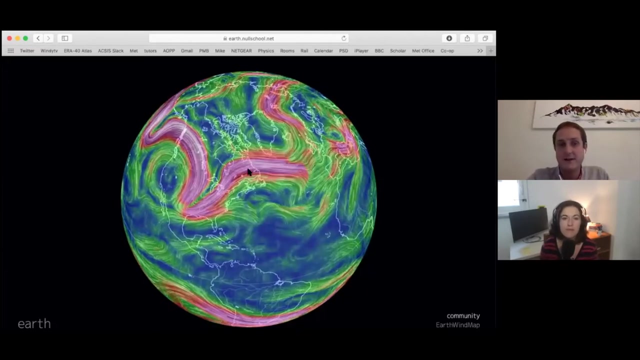 lines indicate the winds. So you can see the this band of very strong wind that's blowing from west to east, So from North America towards Europe, And this is, this is the jet stream. Okay, so if we have a strong band of wind here, and so this is, this is the jet stream, essentially it's a strong 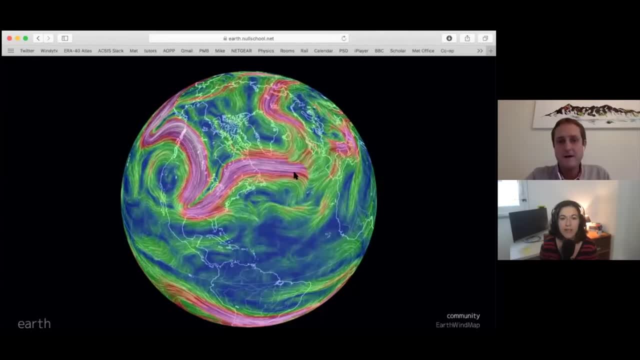 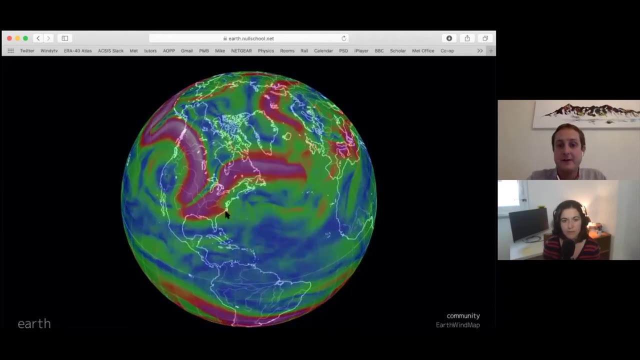 current of wind that blows around the earth, And so you can. yes, right, In what kind of ways can the jet stream affect our day to day weather patterns? Well, yeah, so there's a few things. So, firstly, the jet acts to kind of steer storms and weather systems, So weather systems will kind of 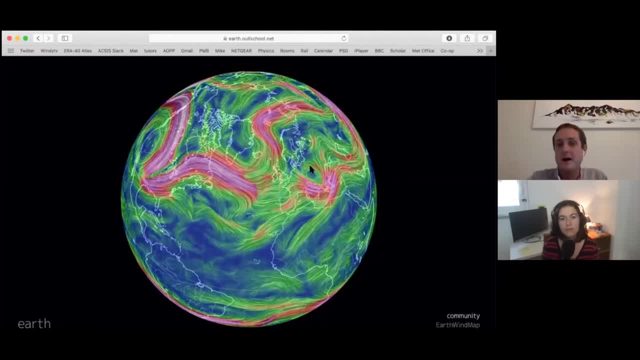 follow the jet and move across the Atlantic into Europe And then the jet will move across the Atlantic into Europe. So a lot of the storms that hit Europe come along the jet stream. But the jet stream can also bring kind of different air masses. So if we think about Europe, the jet is. 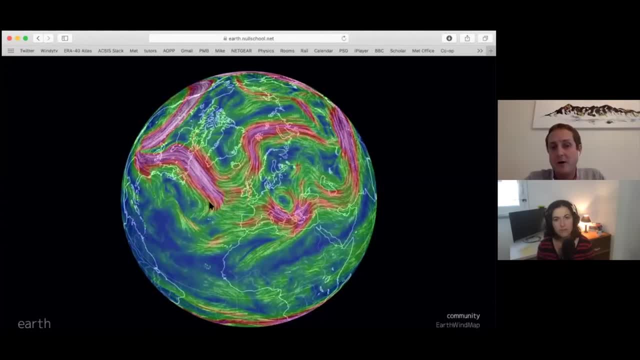 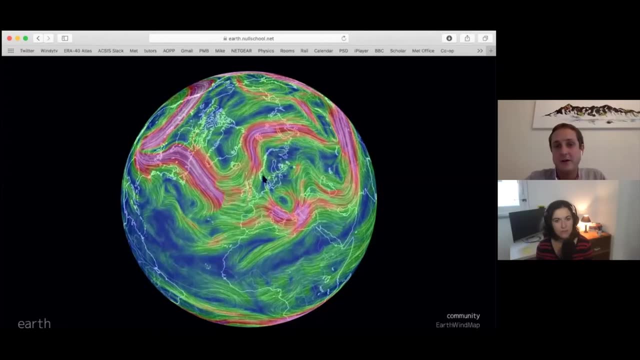 often bringing kind of maritime air onto the continent. So in winter this is bringing relatively warm and moist air into Europe. So it's, this is one of the kind of key features that keeps Europe relatively mild In in winter, And then in summer the temperatures flip around. in the in some of the land is warmer. 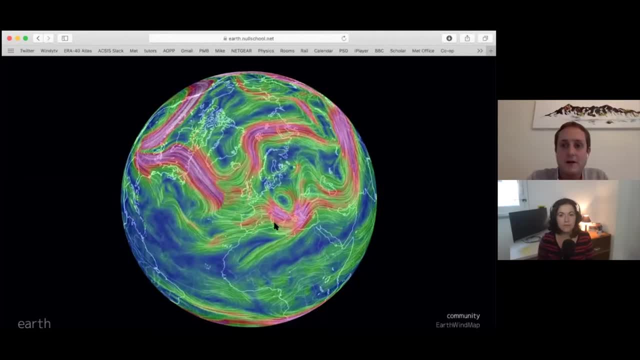 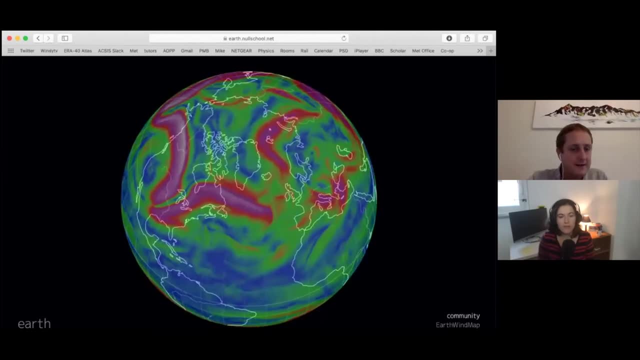 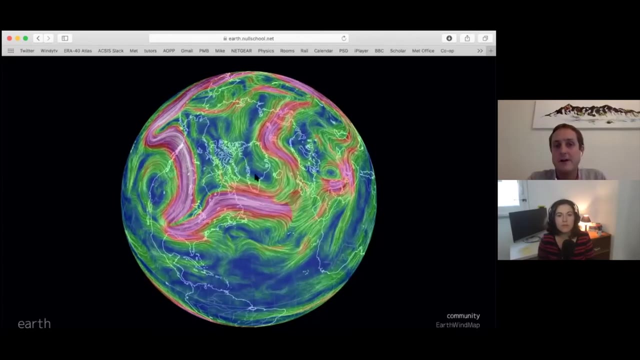 than the ocean, And so the jet is bringing a kind of a cooling, cooling wind from from the ocean. The other effect of the jet has is that kind of marks a boundary between between warm and cold temperatures. So up here in the Arctic we have kind of relatively cold air mass, whereas here in 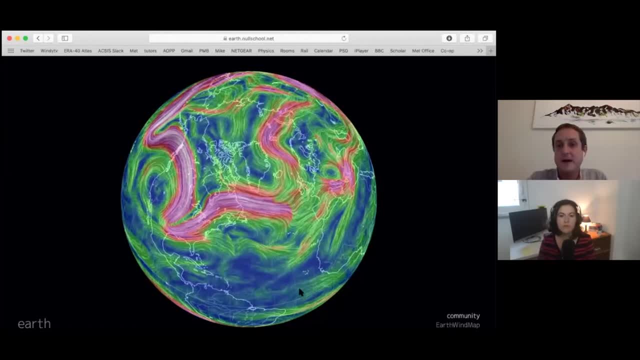 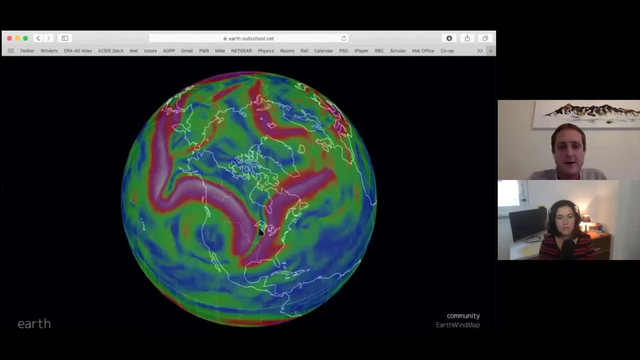 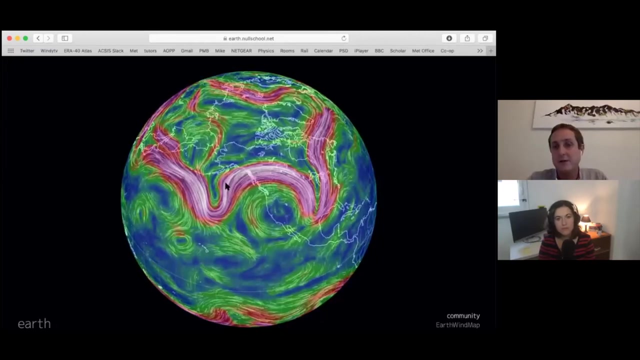 the Arctic we have a warm air mass And so, as the jet kind of snakes around like it does, then this kind of changes which which regions of the atmosphere are warm and cold. So if we look at the moment, there's a, there's a great wave over the north, south and north, like this. This is called a Rossby wave, And 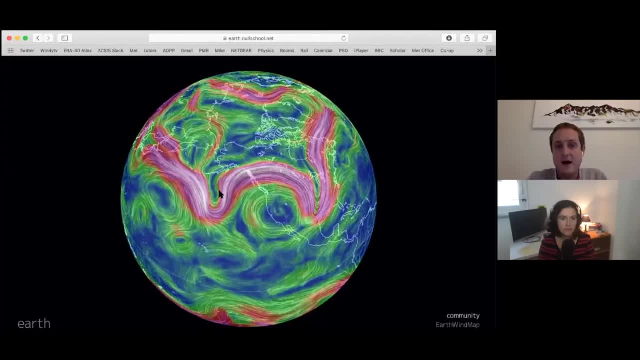 you can see, there's a big mass of cold air here out over the ocean, Another huge area of warm air here over North America And actually these are the conditions that are helping to sustain the California wildfires at the moment, because this will be a kind of a relatively warm, dry normally. 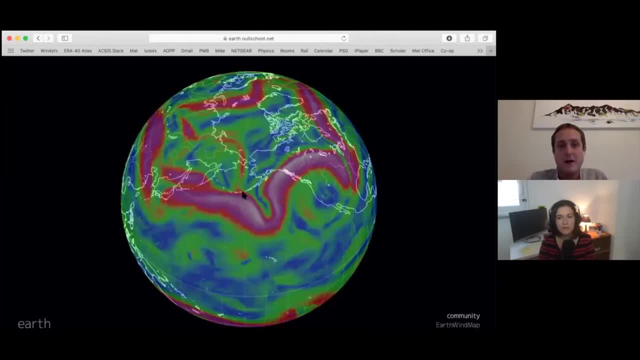 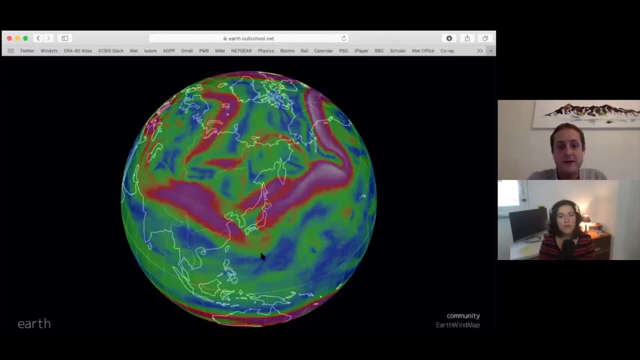 So the jet, really, you know it snakes all the way around the world And it has, it has a huge effect on weather patterns and climates, both in the northern hemisphere. And, you know, if we look to the south, there's a similar, a similar jet structure in the 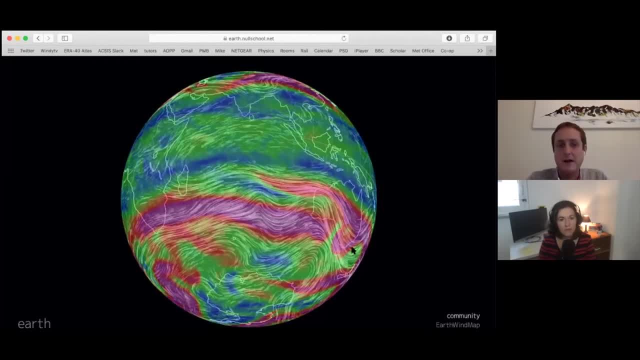 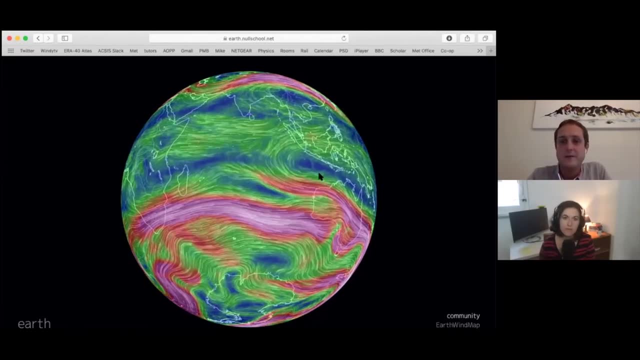 southern hemisphere with these winds going around. So there really are kind of you can see from this that they're kind of the most dominant features. you see, really, when you look at the upper level winds. Yeah, So in your book you actually start. 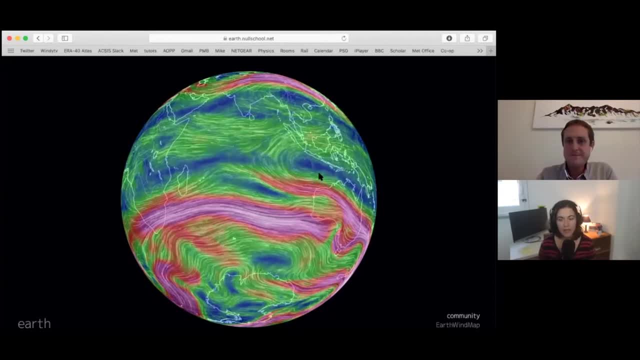 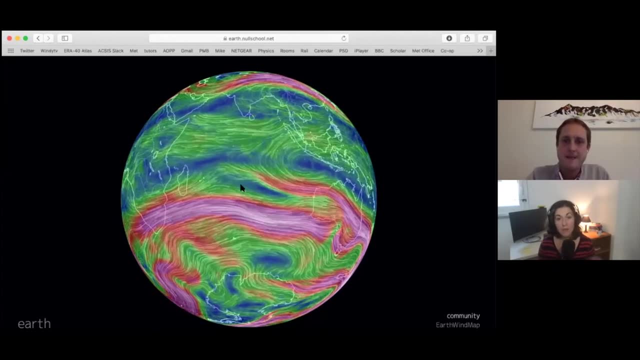 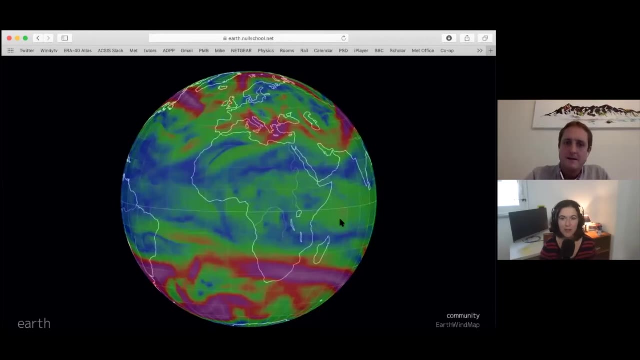 from a story of a weather balloon And this weather balloon basically arises from the Barbados and goes up in the atmosphere and then gets into the jetstream. and I think it's a nice way of you explaining the jet stream, how the winds work and all. 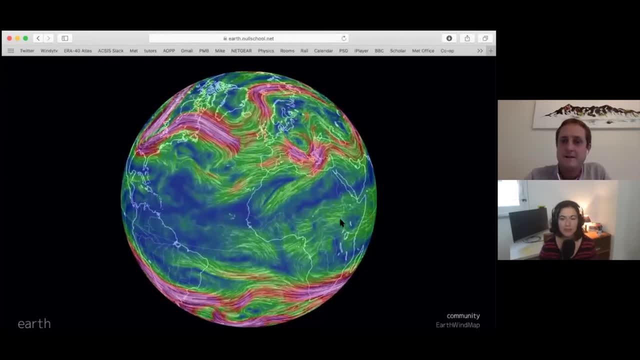 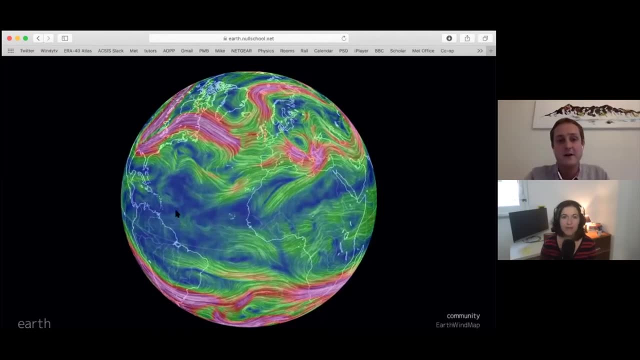 the other effects they have on the climate around the world. Yeah, so I've tried to kind of structure the book as a bit of a journey. So at the moment we're recording this in the beginning of autumn, and so the jet down. 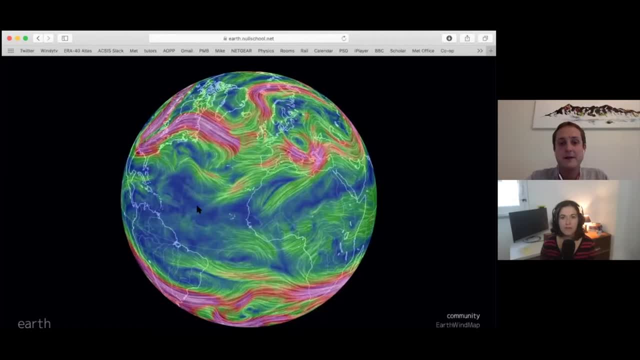 here isn't particularly strong, But as we get into winter there'll be a very strong jet coming kind of from the Caribbean and across Africa here and then across Asia, And you can see a little bit of it now forming already across Asia. 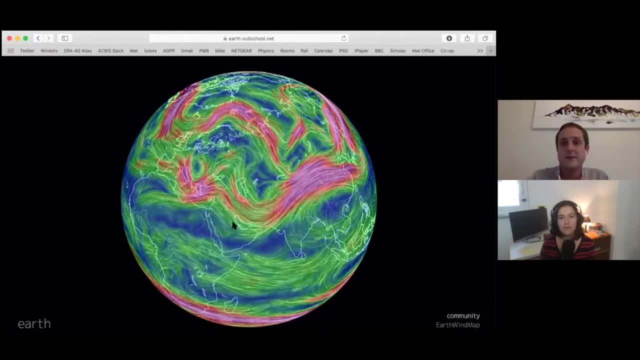 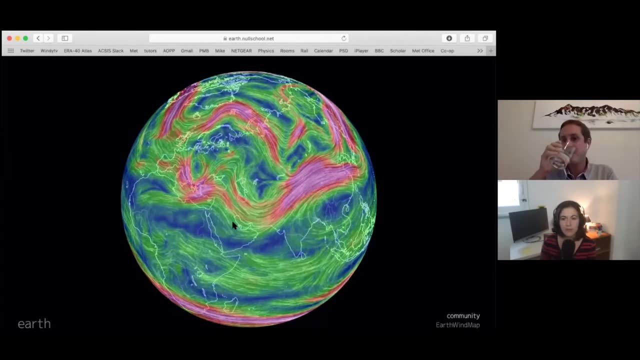 But in a few months' time there'll be a really strong jet, kind of starting all the way back from Barbados, as you say. Yeah, so as I was starting to study atmospheric science and climate, it always fascinated me, Actually two things. 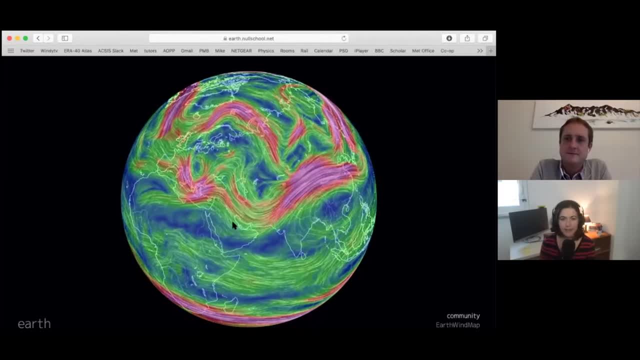 First, how the atmosphere, when you look at it from data- basically not like By eye because you cannot see it, but it really just. It looks like the water, just water movements, a fluid And it is actually a fluid and you can treat it physically as a fluid. 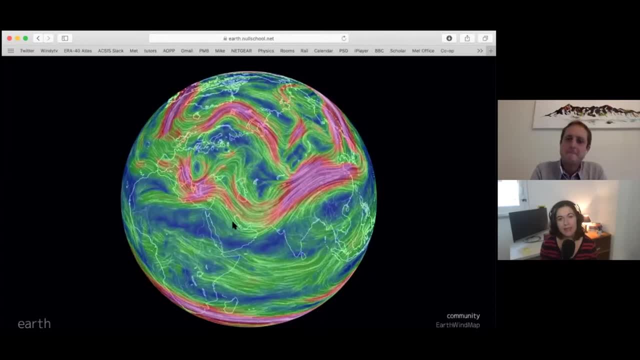 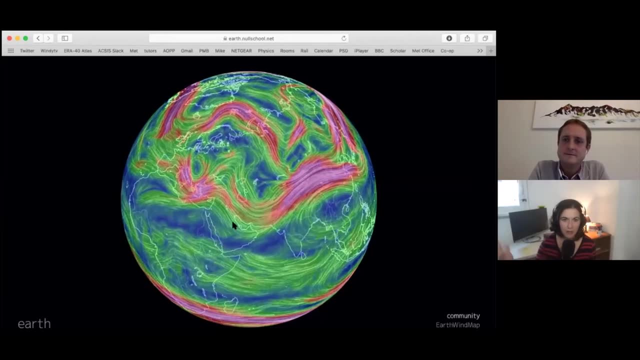 So you explain that in the book as well. And the second thing that is fascinating to me is also how the winds actually get stronger as you go high, And that is, as you explain also in the book, due to the friction with the Earth. 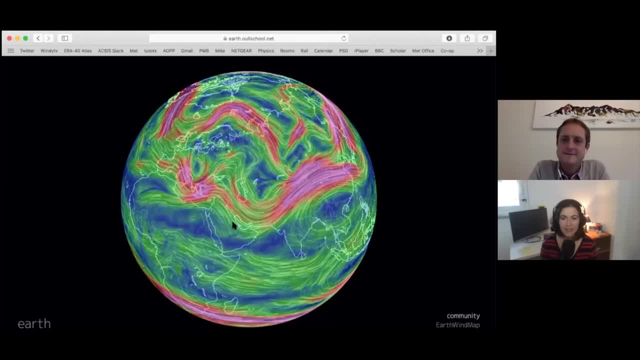 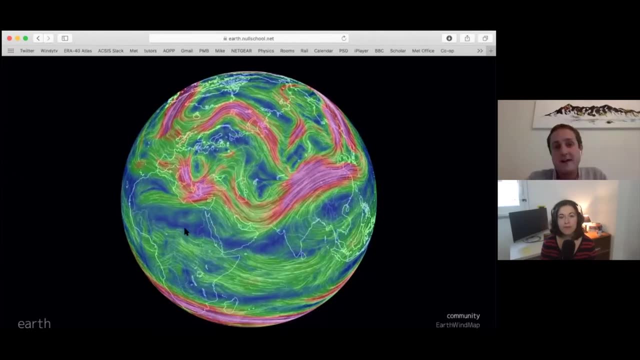 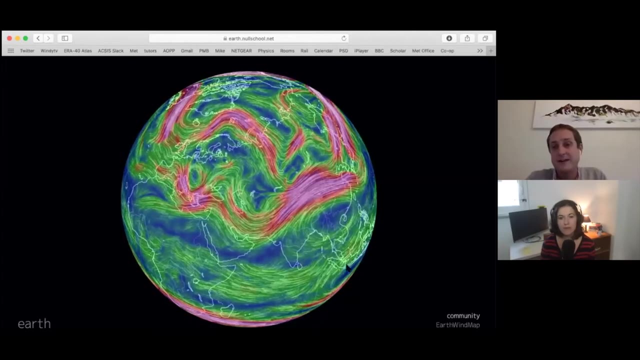 So, yeah, it's really fascinating, Yeah, and there's a few different processes that come together. I mean, essentially, the jets are there. There's a couple of key ingredients why we have the jets. Essentially, we have a lot of solar heating in the tropics and obviously the poles are. 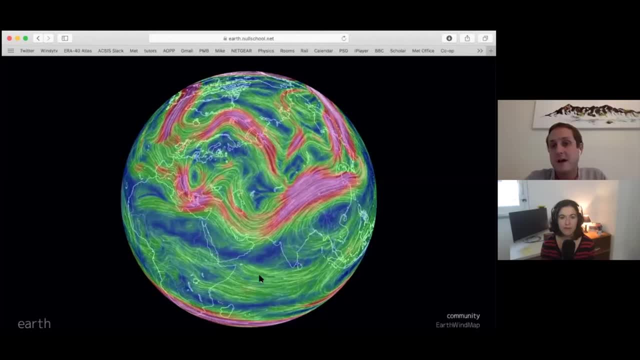 relatively cold, And so because of that temperature difference there's kind of a need for the atmosphere to transport heat around. So the atmosphere has to transport heat from the tropics Towards the poles. So that's one of the key ingredients. The atmosphere has to move to do that. 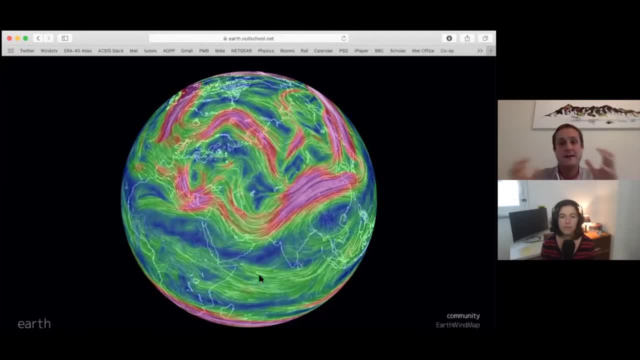 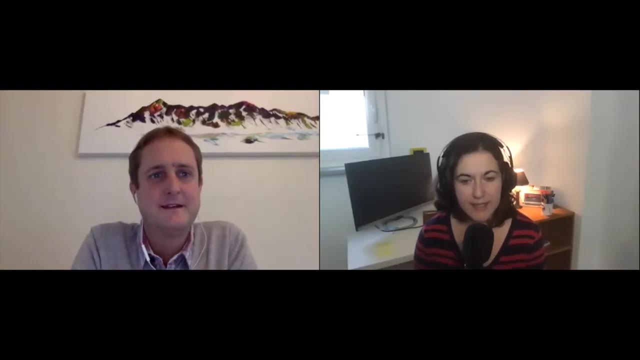 And then because the Earth is rotating, that really constrains the fluid dynamics, as you say, And that constraint kind of naturally leads to the growth of jet streams, Yeah, So something really interesting also that is in your book is that you do a sort of historical 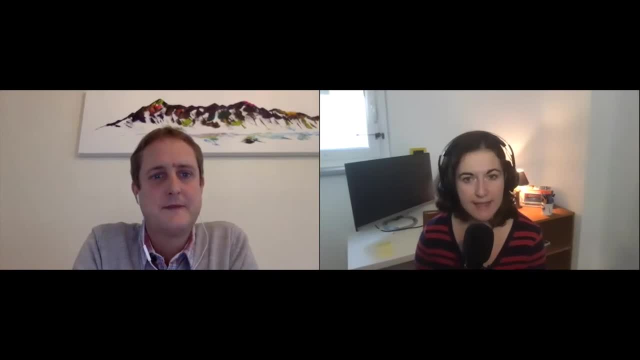 recount of how philosophers, Scientists, already back to the time of Aristotle. Is that how you pronounce it? Sorry, I always studied this in Italian, So the pronunciations are not always like. The pronunciations are not so obvious to me sometimes. 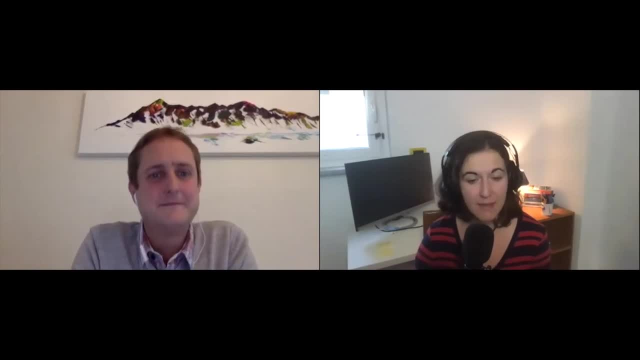 But yeah, how, already then back in ancient Greek- basically we're thinking about weather patterns- and tried to give some first rudimentary explanations for them. And yeah, so it's, Maybe you can, Maybe you can talk a little bit about these excursives that you do in the book. 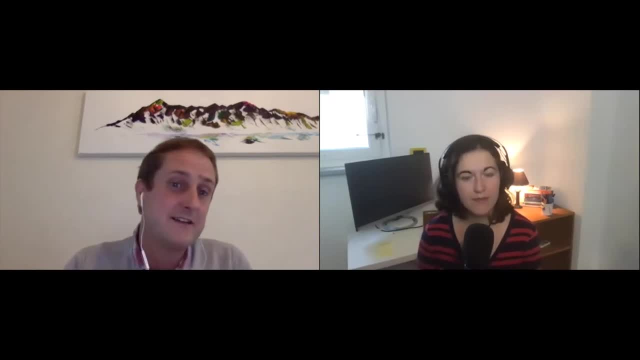 Yeah, So Aristotle had quite a few ideas about weather and about meteorology And in fact he's often kind of credited as being the start of meteorology as a science, Of course. so in general Aristotle had lots of good ideas, but his ideas about the weather 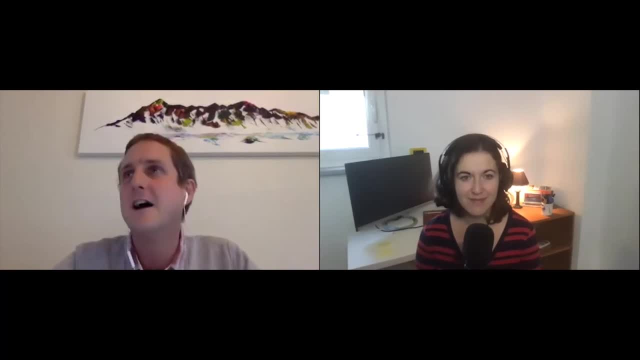 were a little bit funny with hindsight. He talked a lot about kind of exhalations from the earth and the weather being controlled by kind of vapors, some of which you can see and some of which you couldn't see, And so Aristotle had ideas that actually lasted for many, many centuries. 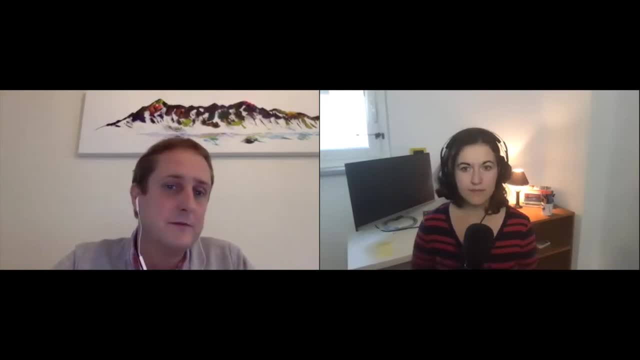 So even when Columbus was setting off on his kind of voyages of discovery, they would still use Aristotle's ideas as a kind of a guide for understanding. And it wasn't actually until just a couple of centuries later, so in the 1700s, when people 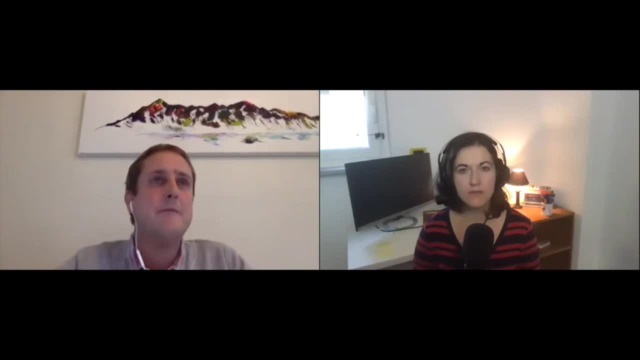 really started to kind of think a bit more logically about what might cause winds and why in particular. why we have the trade winds, So coming from the mid-latitudes where we have kind of changing weather all the time, when Europeans first discovered the trade winds, which were very kind of steady winds, 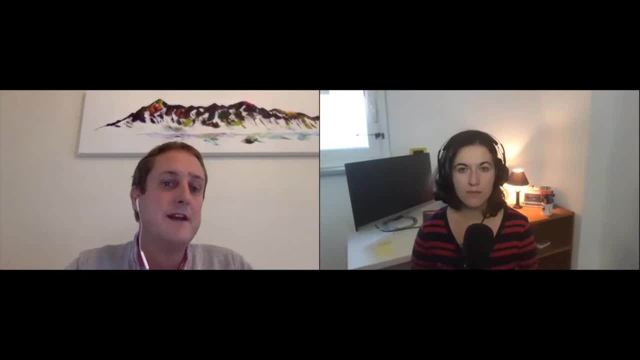 basically doing the same thing every day. that really kind of provoked them to try and understand those winds. And actually it was a guy called Hadley, who was a lawyer in London, who ended up coming up with essentially the correct idea for why we have wind patterns like the trade winds. And it's exactly due to the rotation of the earth and the fact that the warm air that's moving away from the equator is deflected by the rotation. So it took quite a long time after Aristotle before people really got the right idea. 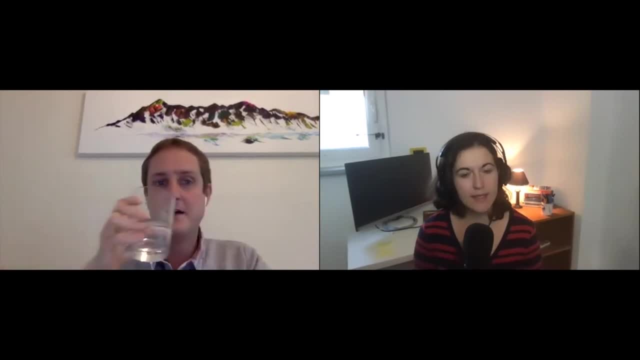 And it also took longer to have a systematic pattern of measurements or like a system of observations that would be able to provide or start what we call now modern forecasts- And if I remember correctly, then you can add to that. but it was motivated basically by wars. 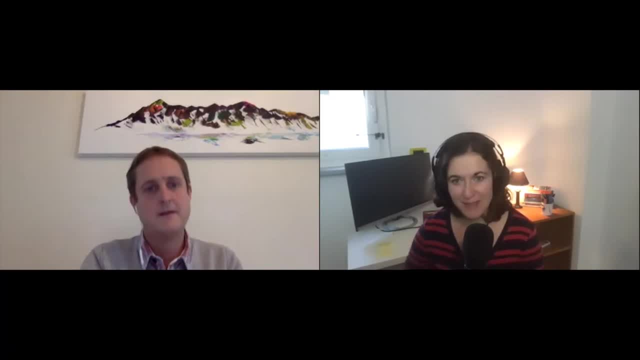 that people. I don't want to know the best routes to attacking other countries. right, That's right. Yeah, So the First World War, I guess, triggered some of the earliest attempts to kind of systematically measure the weather. So particularly in Norway, there was a very kind of active group there interested in applying 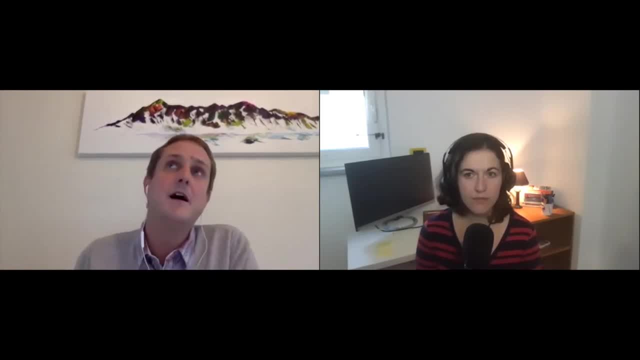 starting to apply. So the first thing that they did was to try to predict the weather kind of the science of maths and physics to the weather. and the war prompted them to really compile detailed measurements of the weather across Norway to try to kind of predict it a little bit better to help with the kind of wartime manoeuvres and things. 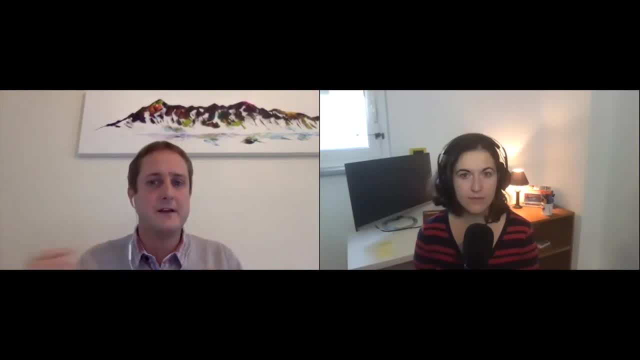 And so those. that was the first time that people started getting good pictures of things like storms, because there was a network of observing stations to observe the weather. But even that was that was only kind of measuring the weather at the surface, And so we've said that the jet stream is in the atmosphere. And so it was the Second World War actually that triggered people to really study that a bit more. So people had discovered very strong winds at upper levels by launching balloons and things, But it wasn't really widely known until the war, essentially when there were kind of high altitude planes in the Second World War. 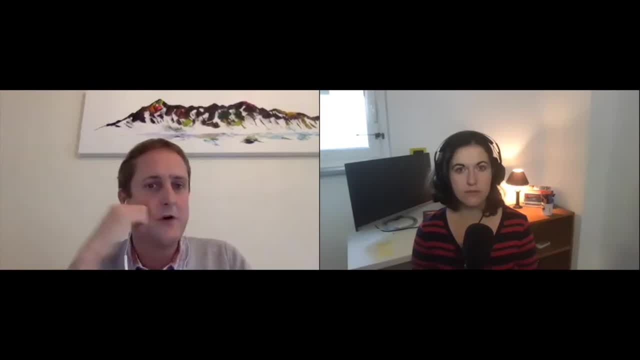 And these would suddenly encounter very strong winds at upper levels which really kind of blew them off course, And so that kind of triggered the need for really studying and understanding the wind patterns, you know, high up in the atmosphere. Yeah, so maybe the only one of the few positive outcomes of wars, I guess. 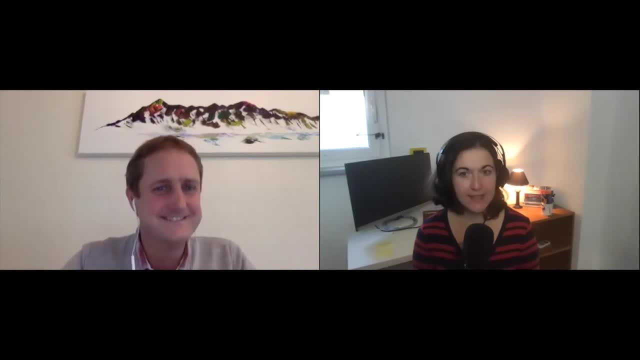 We started looking at these important weather patterns, And this is becoming increasingly important now that we have global warming, And so I really like in the book how you treat the topic of climate change and how it can affect the jet stream and, in particular, 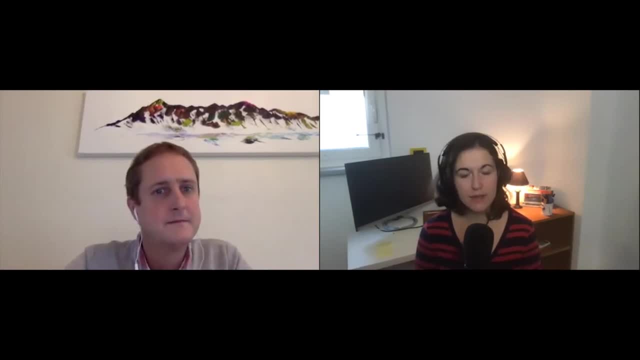 how it can affect the risk for certain events to happen more often. So I was wondering if you could comment a little bit on that, especially what are the expected changes that we can get from the effect of climate change on the jet stream? Yeah, so we do expect climate change to affect the jet. 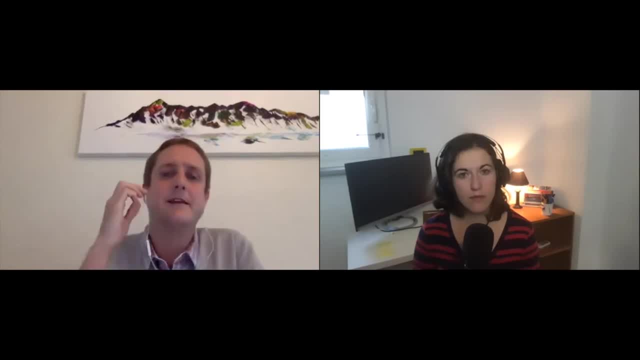 But there's a lot of kind of competing effects going on which makes it quite a tricky thing to predict. So climate change is quite kind of multifaceted. There are several different aspects of it which kind of affect the jet. So, for example, as the 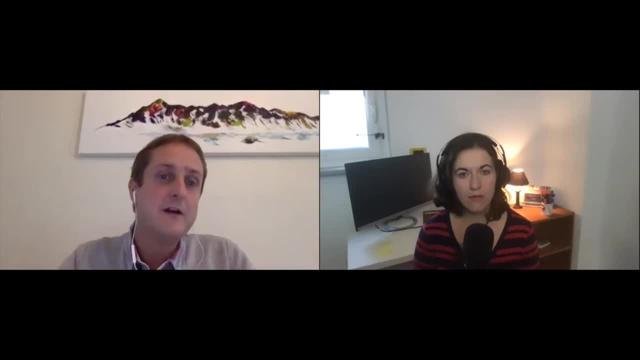 as the air warms then it holds a bit more moisture and so the fact that the air is moister can affect the jet in terms of kind of the distributions of rainfall and latent heating and things. but two of the kind of biggest things are related to the kind of structure of the 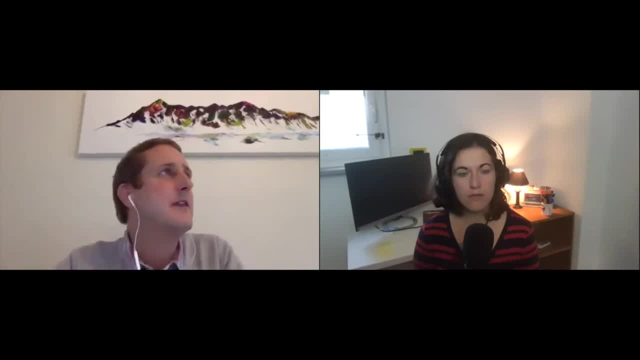 warming. so it's it's quite familiar that the arctic is warming very rapidly. so if we look down at ground level, then the arctic is warming a lot faster than than everywhere else. and we expect this to affect the jet because, as we said, the jet kind of marks the boundary between the warm and the cold air masses. and so if we're, if we're kind of preferentially warming the arctic, then we're we're kind of upsetting that balance between the cold air on the poleward side and the warm air on the tropical side. so if it was just the if it was. 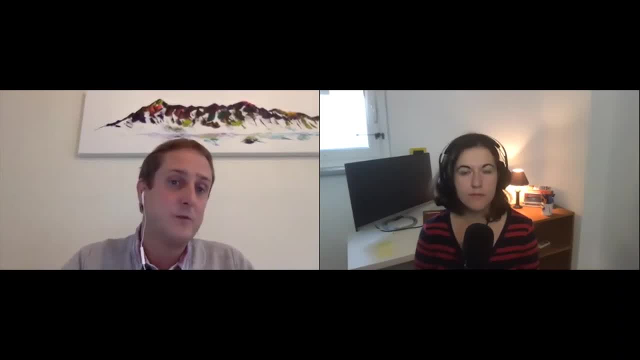 just the warm air on the tropical side, then we're kind of upsetting that balance: arctic warming on its own. we would expect that to weaken the jet and to push it a little bit towards the equator, and that's reasonably well understood. but the the tricky thing is, at the same time the tropics are. 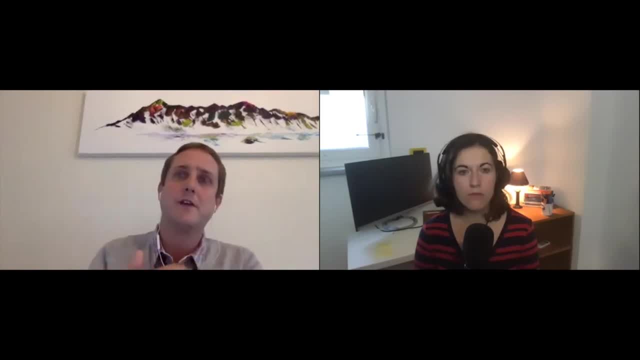 are warming but they're not warming strongest down at the ground, like, like the arctic is. they're warming the strongest actually up at jet level. so if you go 10 kilometers up in the tropics, that are warming the strongest and that's. that's to do with the kind of moisture. 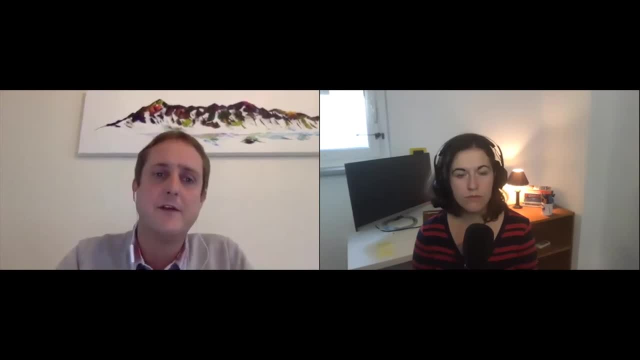 levels in the tropics and the structure of the atmosphere there. so at upper levels then you, you kind of have a force pushing back the other way, so that the, the tropics are warming most and the arctic is warming a little bit less, and so that's kind of strengthening the 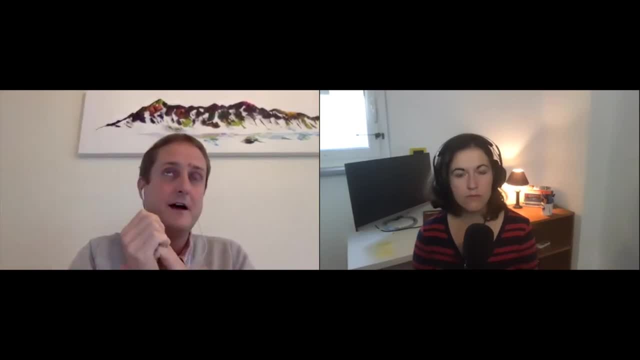 temperature contrast across the jet. so we expect that to push back the other way to, to kind of strengthen the jet and push it a bit closer to the poles, so we kind of have this balance. it's not it's like a tug of war, but they're pushing, so it's. 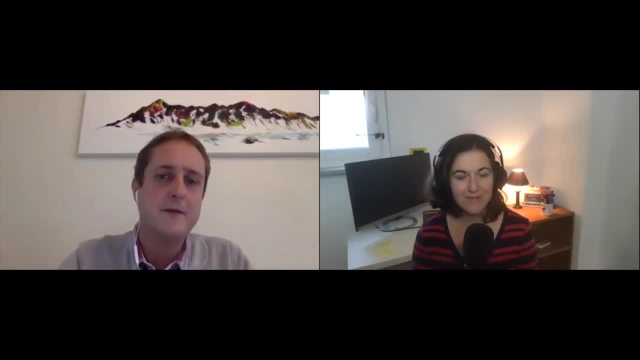 it's more like a kind of push of war, uh between the, between the arctic and the tropics, uh, and we think um. so, just based on on our, on our kind of best models, uh, best computer models, today it looks like the tropics are going to win that battle, um, but there is a lot of uncertainty there, um and if? 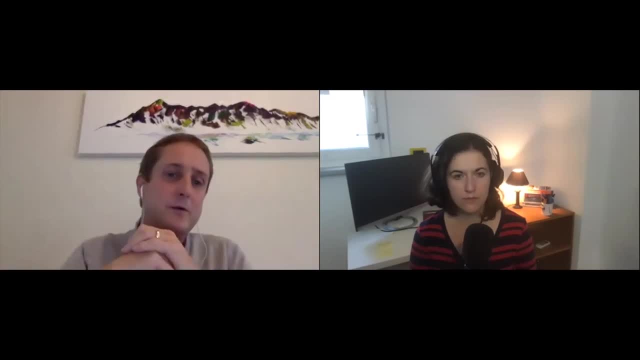 you know, because we've got the the battle between these two competing forces, um, you know, often the changes predicted in the jet are relatively small. um, but if any of these you know, if either of those two are kind of wrong in the models, then we could see bigger changes than than we're predicting at. 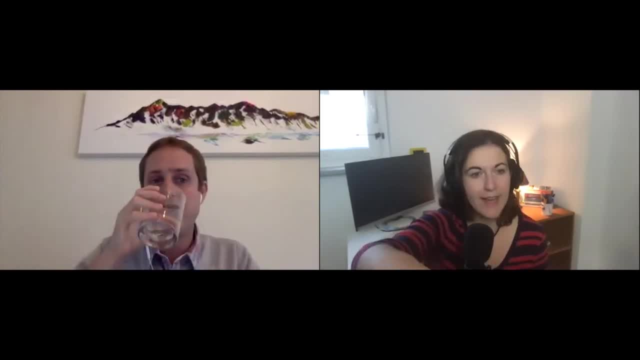 the moment cool. um, if i can, i have an excerpt from the book that i found particularly interesting and inspiring, especially as a scientist, uh, regarding communication of climate change. so, uh, if i may read it, um, and then i would ask you to comment on that as well. 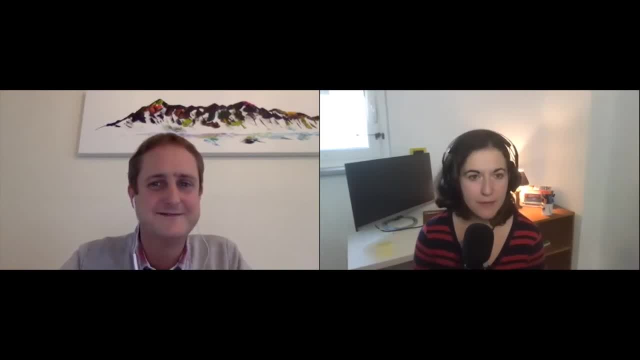 um, all right, so i'm gonna go ahead. this is front page 188, so, and it goes. uh, climate scientists used to use to issue a blanket response to this question, and the question is related to: how does climate change affect the jet stream? uh, we can't blame climate change for any individual. 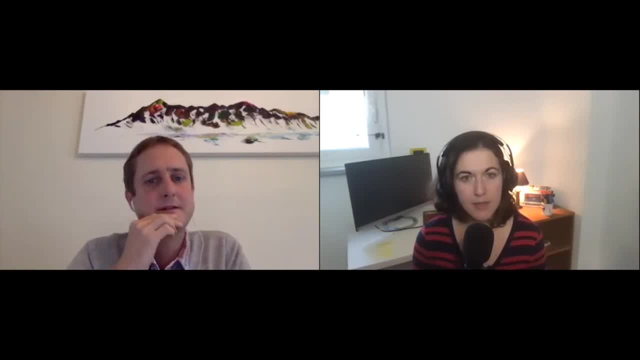 event. climate is some carefully defined average state, albeit a changing one, and individual extreme events are weather which is different. but it's becoming increasingly clear that we can and should say more than this. the way to do this is to resort to probabilities and consider how climate change. 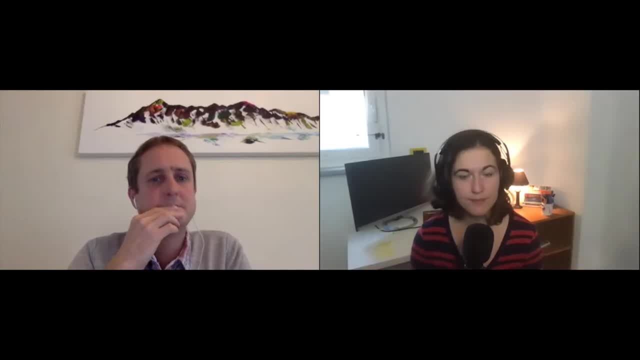 has halted the risk of certain extreme events. um so yeah, i found this particularly inspiring because it is true at least 10 years ago. climate change has halted the risk of certain extreme events. um so yeah, i found this particularly inspiring because it is true at least 10 years ago. 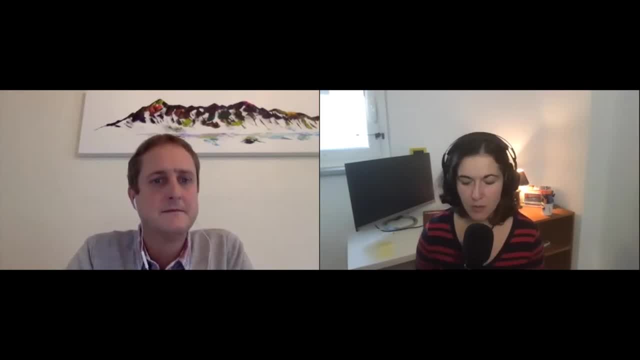 when i started my phd that we had this, this sort of default answer that, um, you know you can't attribute a particular event to climate change, but over the course of these last 10 years, i think, uh, we have witnessed a lot of extreme events and we have done research, uh, to demonstrate that the 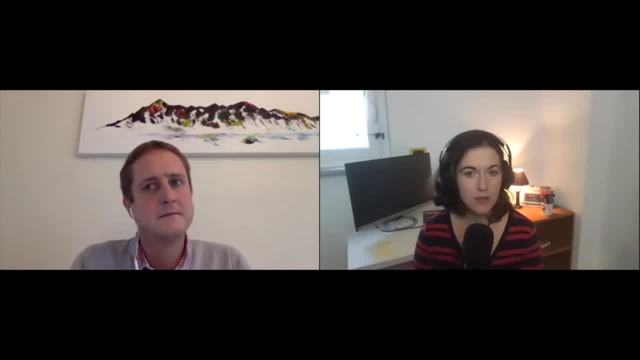 probability of these events has actually increased, or and is it going to increase even more? uh, with the way that climate change affects climate change and the way that climate change affects climate warming on the earth, yeah, so, um, uh. so, as you say, we um. a lot of the time we used to just say, oh we, you know, we can't. 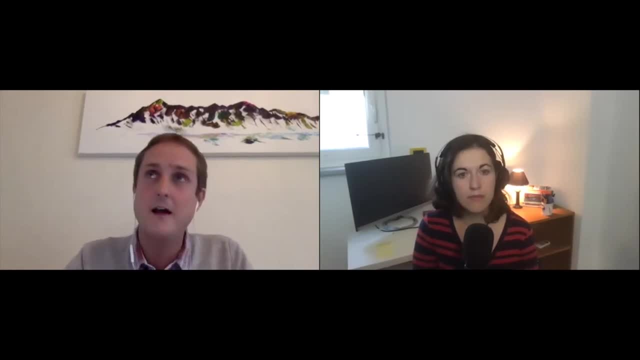 really comment on individual weather systems, uh, and there were lots of analogies, so things like, um, uh, we often used to talk about, about rolling a dice, like if you, um, if you have a normal dice, uh, and then you, you let's say that you load it somehow so that it's more likely to throw a six. 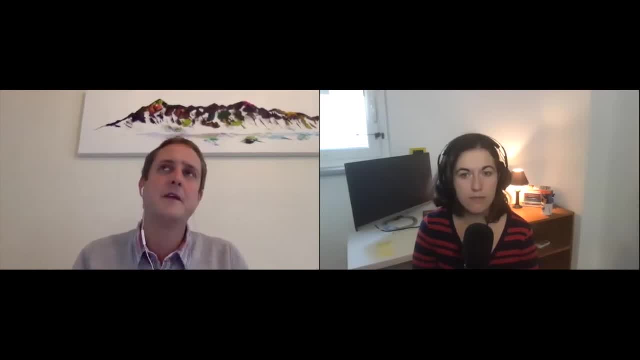 um than than just a regular dice. um, so if you, if you roll your loaded dice and you and you get a six, um, then how do you, how do you interpret that? do you uh? does it make sense to ask if, if you got the six, uh, that particular six because the dice was loaded, or uh, or might you have got that six anyway? 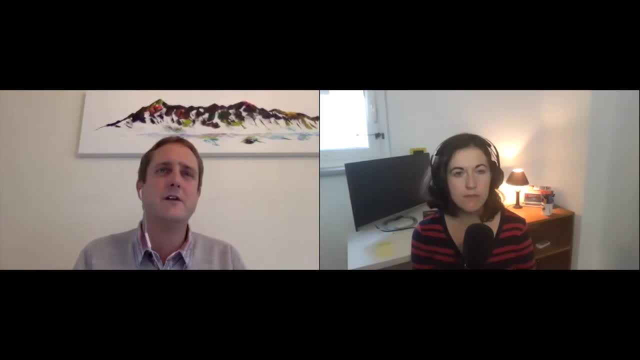 um, uh, it's, it's kind of a it's not. it's not obvious that the question makes sense: um, so it's, um, so, yeah, it's. it's generally better to to kind of resort to probability of events. um, so i think we have to have more probability of events for different opportunities when we talk about this. 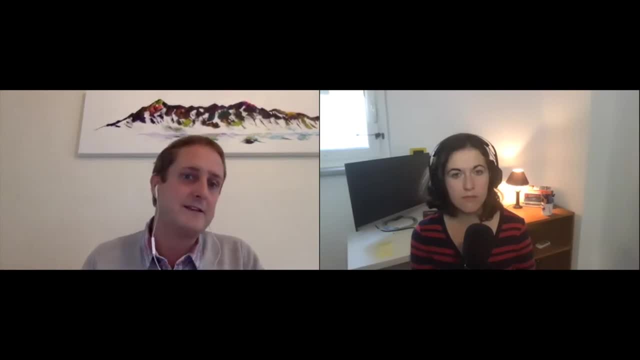 thing and say, in that case we'd say, well, loading the dice has has changed the risk, um, it's changed the probability that we'll get a six. um, uh, and that's that's generally how we approach extreme weather events. uh, these days, um, and you're right that we often, we often do see these things first. 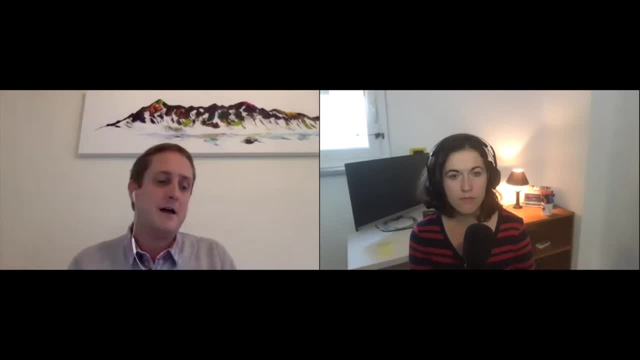 in extremes, uh, we'll often have an extreme event, uh, whether it's a flood or a heat wave or something um, and in explaining these, these, these events, we increasingly need to include the fact, the effect of climate change, um, uh and so. so, for example, if you think about, about a heat wave, um, so let's say: 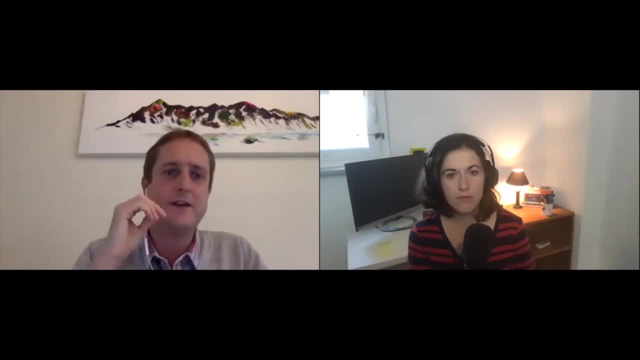 let's say, for the sake of argument, a heat wave happens when you get over a certain threshold. let's say, let's say, 35 degrees, uh, um celsius, um, uh, maybe in in a, in our kind of normal undisturbed climate, maybe that kind of event maybe is quite rare. let's say that happens. 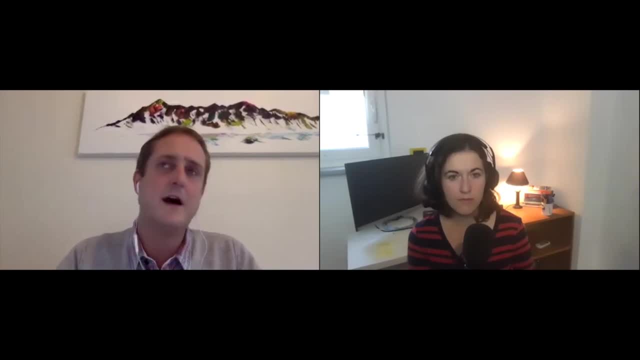 you know, one every 20 or 30 years or something. um, if you, if you make a kind of a small, a small kind of average change, if you warm the whole climate, say by one degree, um, i mean that's a fairly small change. if you know if the difference between a hot day and a cold day is, you know, is, 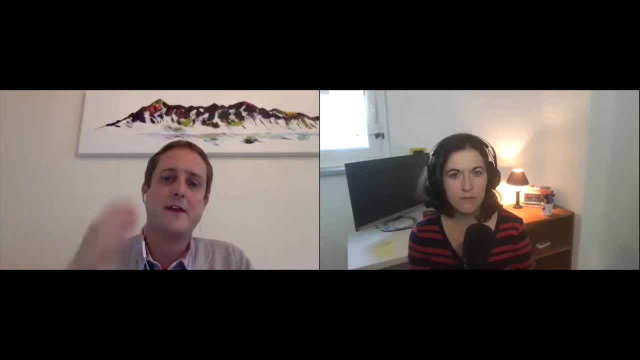 is 10 or 20 degrees or something, then, uh, then you might think, oh my, my one degree isn't going to make much difference. um, uh, but actually that has. that has a really big difference on the, on the extreme events, at the tail of that distribution. um, so just warming. warming the whole distribution by one degree, um, uh, can actually lead to a really big increase in the in the risk of having those heat wave days, um. so so suddenly you might find that your, you know your heat wave days, they're not happening every 20 or 30 years, they're happening every every five or 10 years, um, and that's the kind. 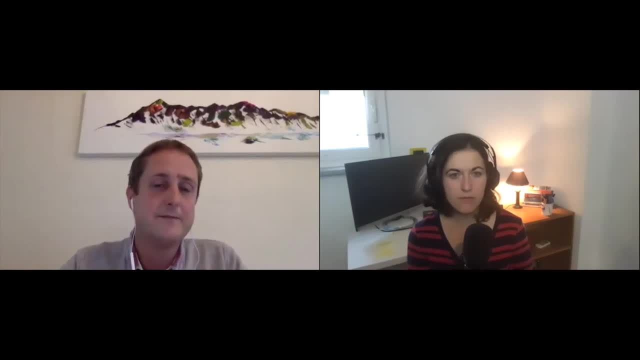 of thing that we really notice when we have these, these extreme events, cool and uh. so there is also a lot of talks about the, say, temperature targets, um, like the paris, paris agreement of um reaching 1.5 degrees celsius warming, but um, you know something that is not much talked: 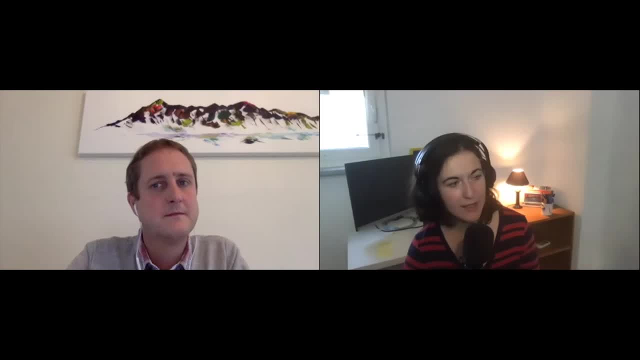 about or not like, at least not as much by um climate scientists to the public is that? um, a lot of these things are also non-linear, as you said. so if we it's not like, if that, if we exceed the 1.5 degrees and we go to 2.5 degrees, we are expecting a sort of like steady, steady increase. 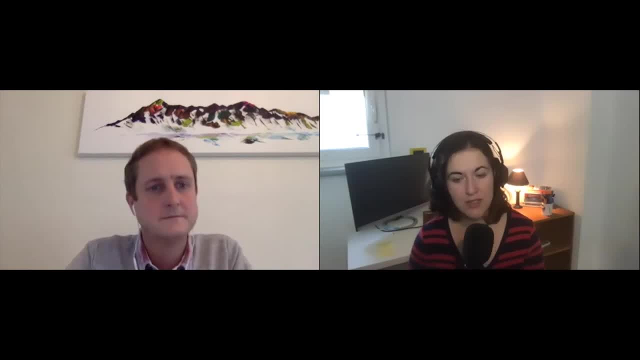 but there, um, there could be more of a much steeper increase and like more of an um much larger number of these extreme events that we talked about. uh, but uh, i'm not too, too familiar with the latest findings in that, so, um, i was wondering if you could say anything about that. 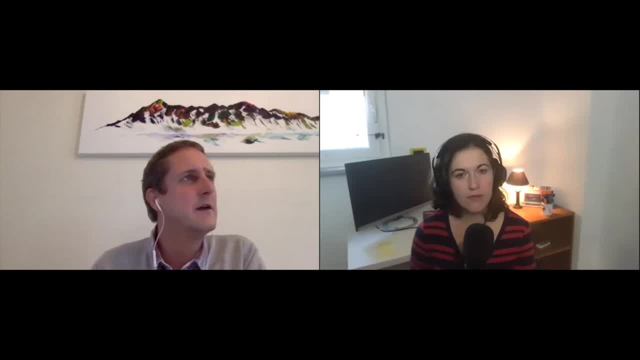 yeah, i know, i know a little bit about this area. i guess, um, the um, you know, the climate system, as you say, is complicated and it's non-linear, which means there are lots of feedbacks. so if you, you know, if you, if you, if you change one aspect of it, then that 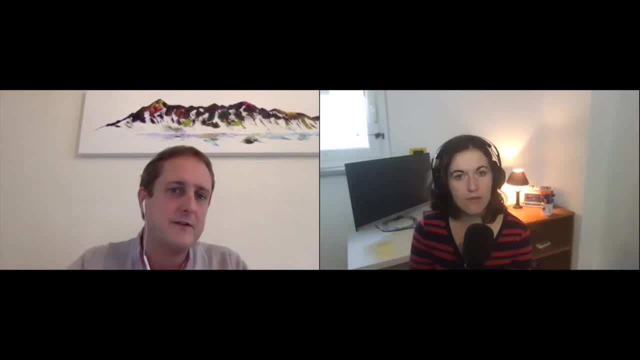 aspect can, can change something else and then it can feed back onto the original um perturbation, um, so. so yeah, we, we certainly can't assume that if you, you know, if you, just if you just keep warming the atmosphere a little bit more, it's not always going to keep responding in in the same way. 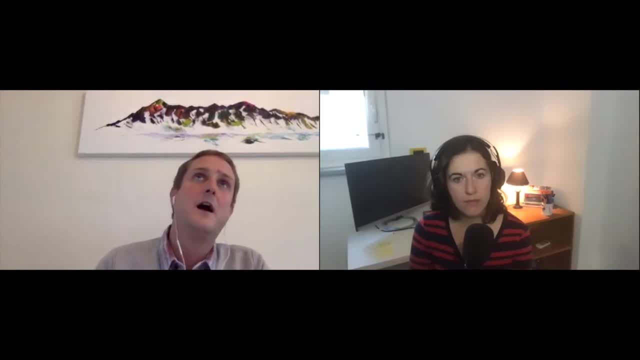 um uh, and so um uh, yeah, there are. there are definitely concerns, as, as warming strengthens, then we have less of a um, we have less understanding, i guess, of of how we're going to react to the climate and we're going to react to the climate and 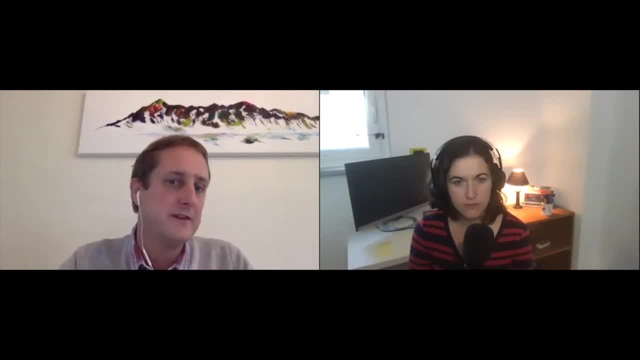 how you know how strong these feedbacks are going to come in and which bits of the system are going to to dominate? um, so certainly the um. you know, if we can, uh, if we can perturb the system as little as possible, that would be a very good thing, i think. yeah, uh, so cool, what inspired you to write? 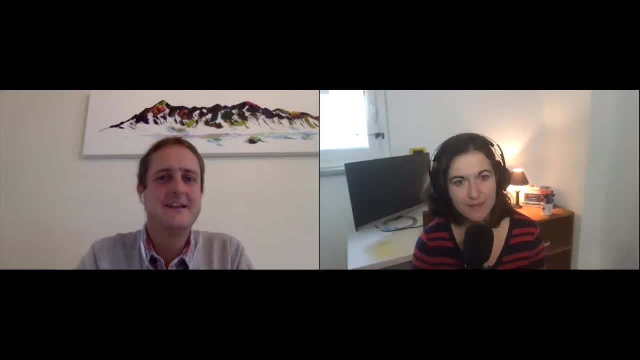 this book? uh, so i think the original motivation was: um, was that people? it became apparent that people were talking a lot more about the jet stream it, you know, it was a lot more about the atmosphere. so it started to feature in in weather forecasts. um, that you'd see in the media, um, and 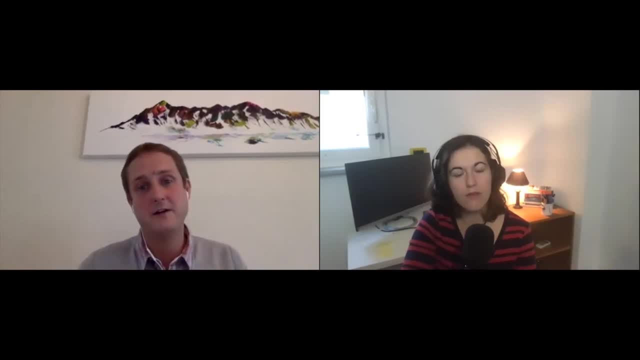 there'll be a lot of debate in the media about the role of the arctic, the fact that the arctic was warming rapidly, and how was this affecting the jet stream? um, so, so my original motivation was to um, was to kind of um, uh, was to talk about some of those issues. um, but the more i uh, the more i. 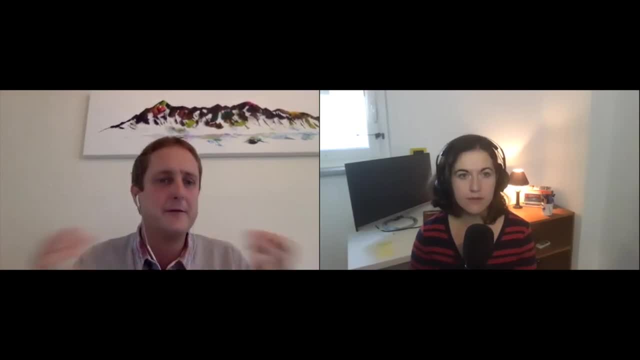 looked into it i realized there's actually very little written about, about atmospheric circulation for, uh, for a kind of a general audience, um. so so some of the history and even just the fundamentals of of why the atmosphere moves and why we have jets, um hasn't really actually been explored very much in kind of the popular science.